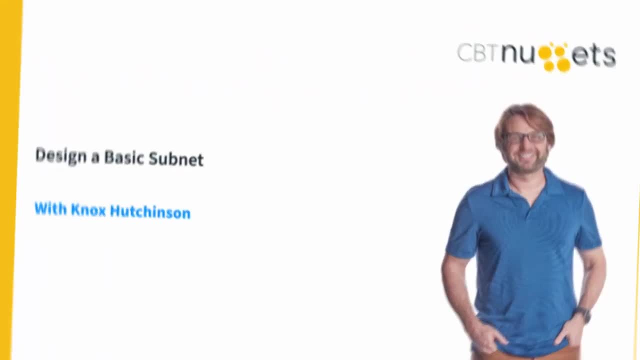 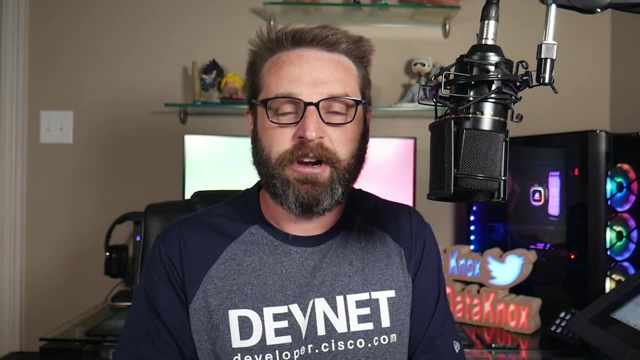 Now it comes time to think real world. We understand how IPv4 works and subnetting works, but what is a real world situation where we would actually have to use it and make a design scenario In this nugget? what we're going to do is we're going to take one network and actually 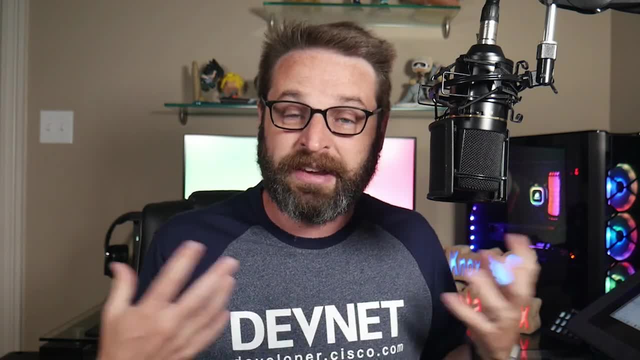 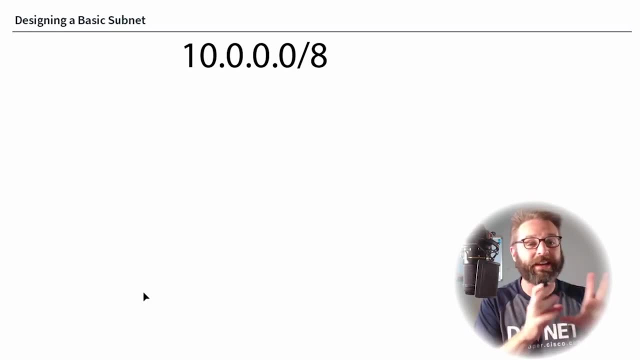 talk about the components that should actually build up those four octets that we need in order to create an IPv4 subnet. Let's get going. So now it's time to actually take those IPv4 skills and put it into action. Here's the thing: When we do this, we're going to be met with constraints. 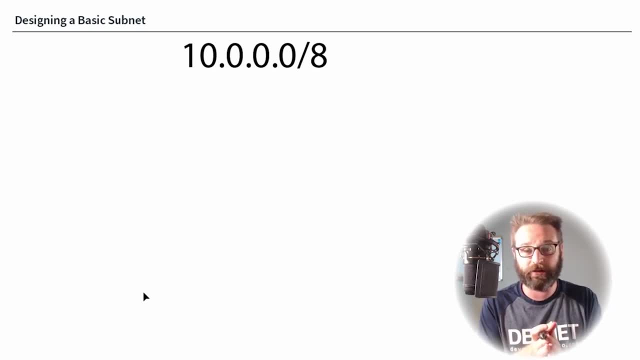 We're going to be met with rules and guidelines about how we should design our network, or at least we should think about what these rules should be. Maybe we're the decision maker on what the rules are. The point is is we can't just throw a gigantic subnet at it and hope that. 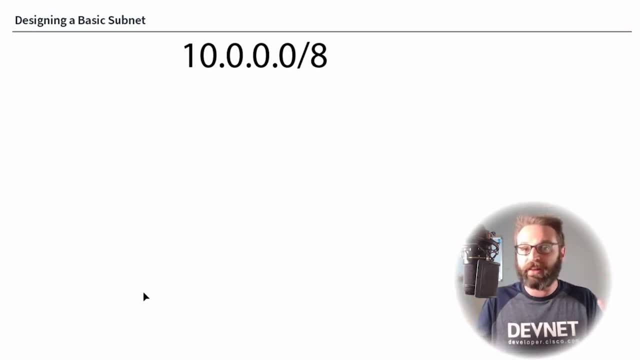 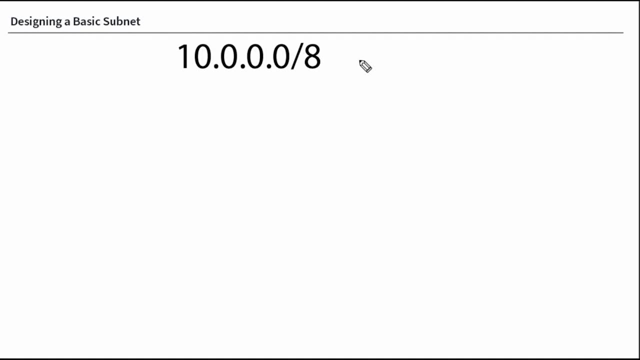 it works fine. We need to think about the future, We need to think about scale, We need to think about stability and we need to think about security. So let's start off with taking the 10 class A subnet. This is 10.0.0 slash eight. 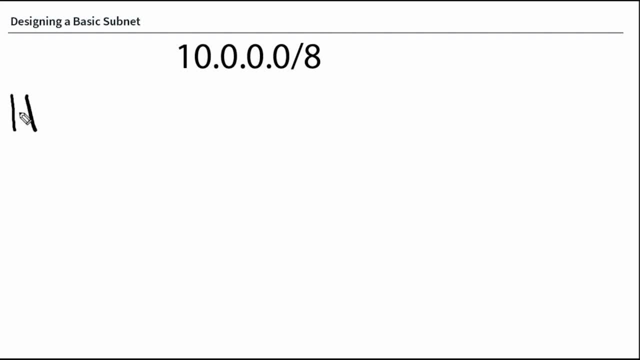 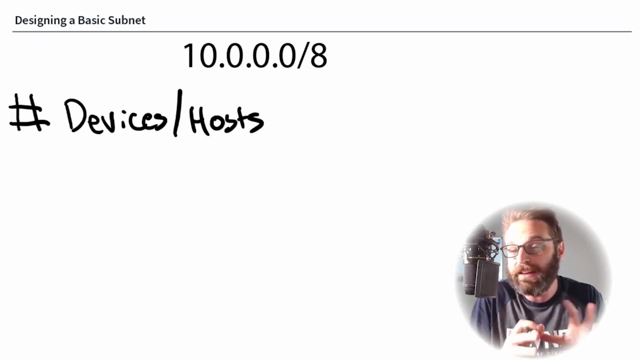 The first question I'm going to ask myself is how many devices need to be connected into this network. So I'm going to put number of devices slash hosts. This may be the most important thing to factor in when it comes to designing a subnet. We need to think about how many devices are need to connect to this network. 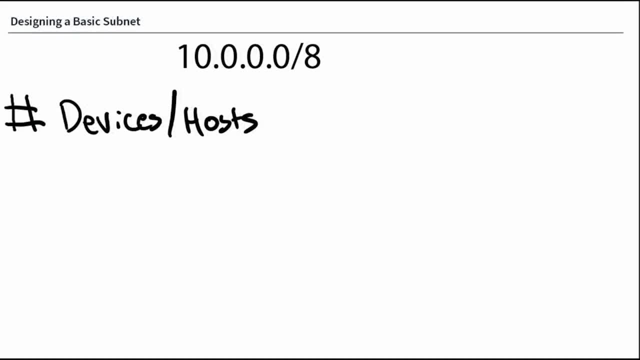 and whether or not they should be separated from other networks. For instance, let's consider for a moment that we have 200 users on our campus, and maybe some of those users have a desktop, Others have a laptop, Almost all of them have a cell phone, and some of them may even 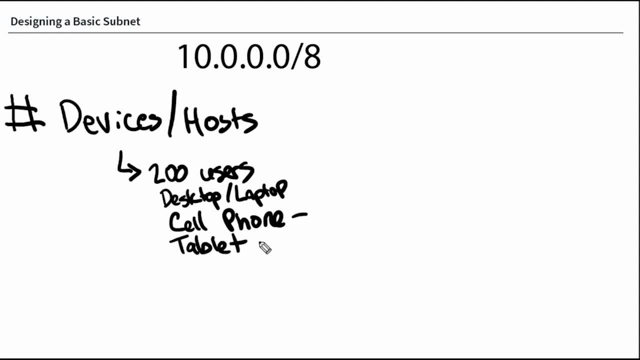 have a tablet. Now here's the other kicker: That cell phone and that tablet are not corporate issued. Those are bring your own devices and we don't control what goes on in those devices. What are they really accessing on their device? What are they really downloading? And this becomes now: 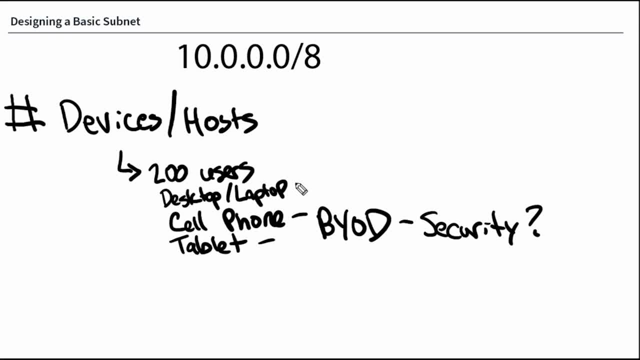 a security question mark right here. So my first question actually goes: do I want people's cell phones and tablets to access the same resources that I want their corporate desktop or our corporate servers to access? And the answer is no. So each user will. 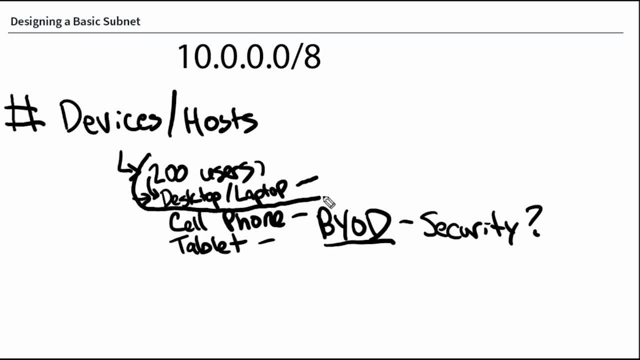 either have a desktop or a laptop, And my first consideration is: this network needs to hold 200 hosts and we shouldn't factor in their cell phone or their tablets. We should create a separate network for that. You can make the exact same argument about IOT devices, which are things like. 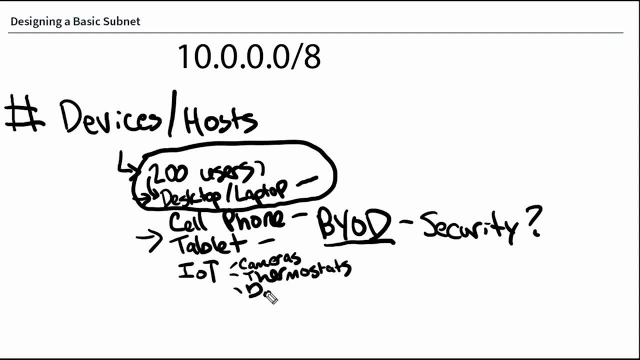 cameras, thermostats- This day and age- doorbells- or card scanners. You could make the same argument about servers and printers. We want all of these to be on their own unique networks. So if I'm only focusing on the task at hand, which is designing a subnet for just the user's data, for their actual 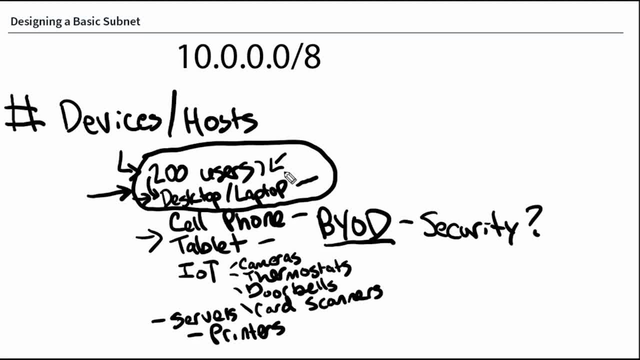 corporate data. I'm focused in on 200 users And this becomes my first subnetting question. We're all pretty familiar with the slash 24, subnet because that's what everyone uses this day and age, And that slash 24 subnet we know. 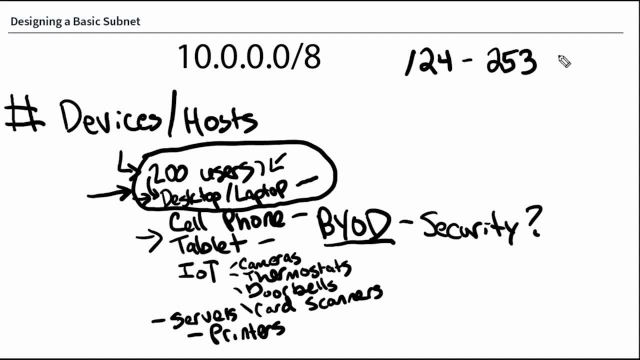 allows 253 hosts, because one of those is eaten up by the broadcast and one of those is eaten up by the gateway. If I were to slide this up to a slash- 25, what happens? The number of available hosts gets halved, really down to 126, because again, one of those is eaten up by the network address and 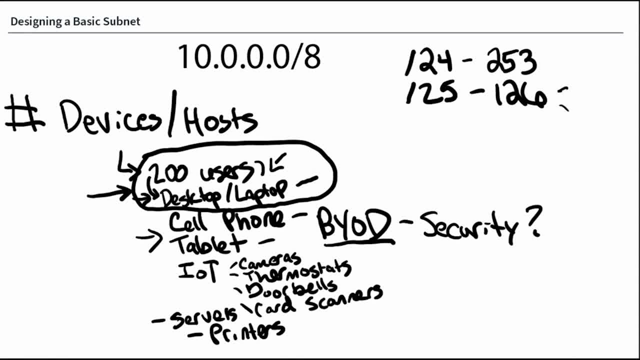 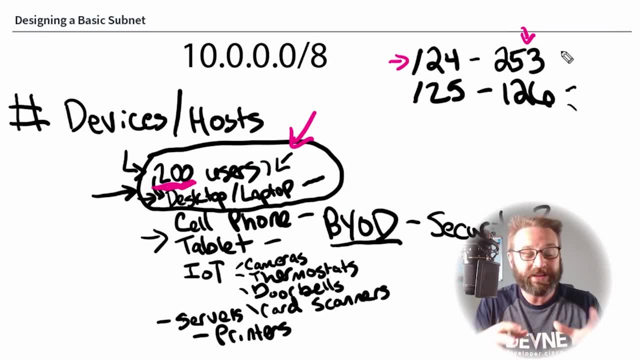 one of those is eaten up by the broadcast address. So a couple good things come into play here when we're actually doing it. First of all, we meet our minimum requirement of 200, but then we have an additional 53 for growing room. This is another very important point is that we want to have growing room. That way, we 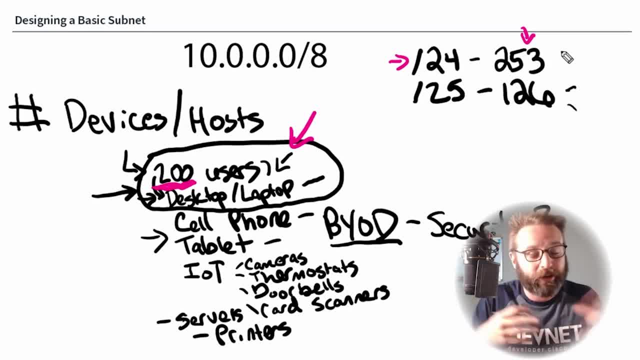 can expand our resources and expand our user group, because our company, we want our company to keep growing, right? That's the entire point- is that the business should keep growing and we should keep hiring. So by doing the design like this, with a subnet like this, we actually have 53 additional. 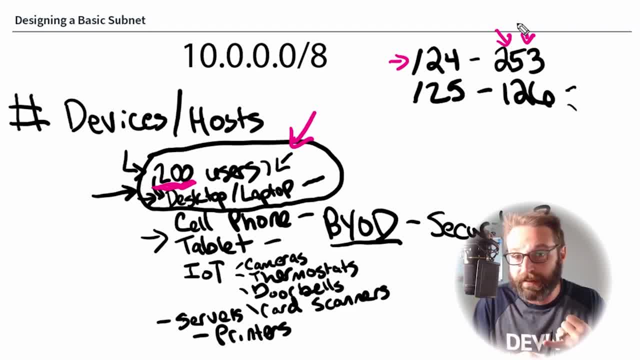 hosts that we can add and that makes it scalable. So we've kept security in mind here, because we're not running all of our devices on one separate sub, on one subnet. We're going to break it out. but we've also got scalability in mind here, because we've got the ability to grow a little bit. This begs the. 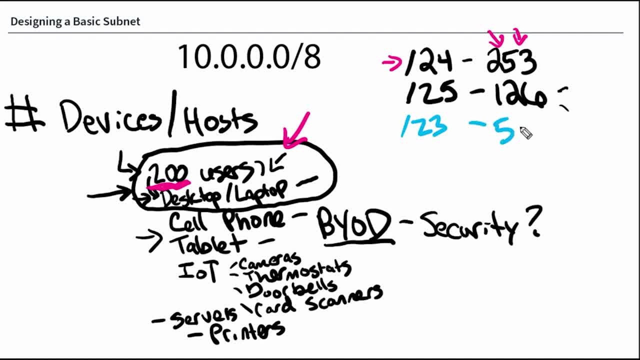 question: Knox, why not just go with the slash 23 and get the 500- whatever devices here? See, I'm so bad at subnetting I can't even think of it. off the top of my head That would be like 510 usable. 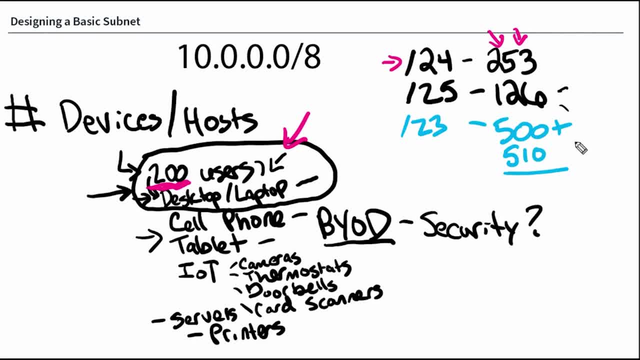 addresses, I think because this is going to be a gigantic broadcast domain and it eats up all the IP addresses somewhere else, We don't expect to add more than double our addressing space in the near term. This even begs the question about stability, Like when we have a broadcast domain. 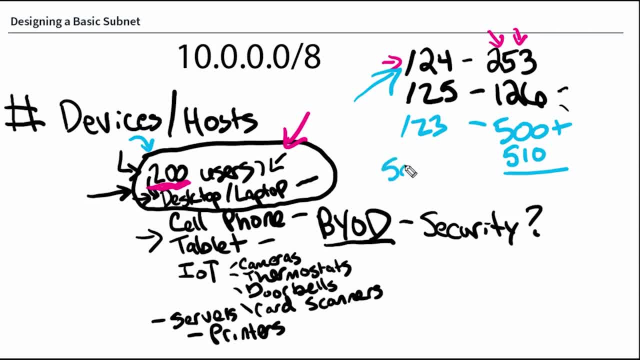 that is that big, when the broadcast domain exists of 500 devices, there could be a lot of broadcast going on and this could actually be a problem And we may want to limit it, especially if we're using legacy hardware that's kind of older and it's processing power and ASICs just. 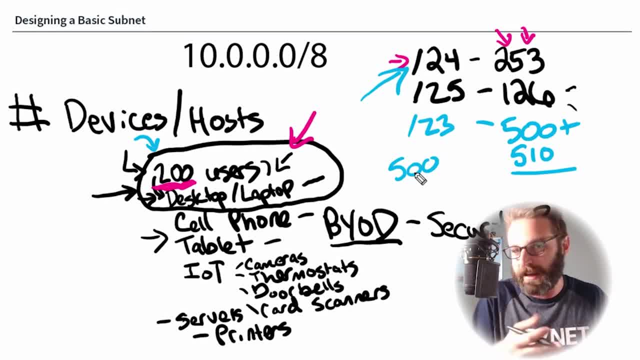 aren't up to snuff the way we want them to be. Limiting the broadcast domain may actually be a good thing for us. That way we control how our switches switch and how our routers route. So with this design of a basic subnet, we now have things like stability. 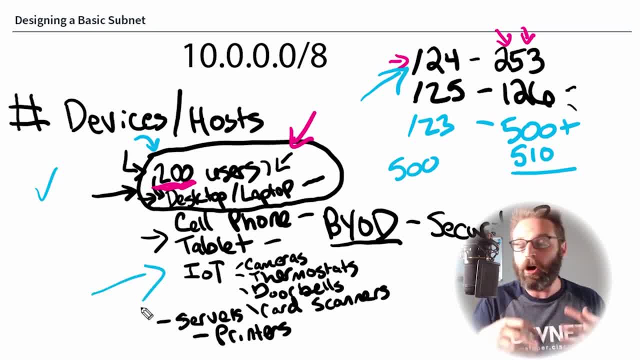 scalability and security in mind. We're separating all of our different devices. That's the first and most important one. We're separating our corporate data from the devices that could be compromised, like cell phones and tablets and IoT devices. We also have met. 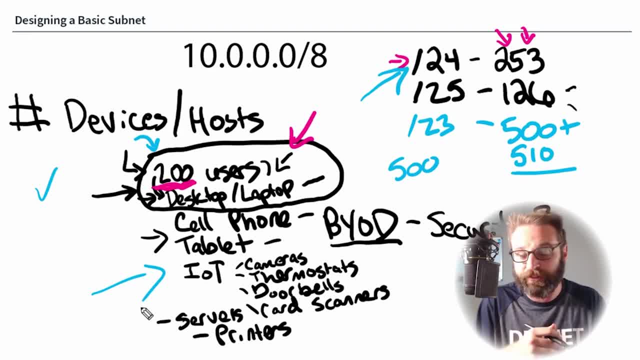 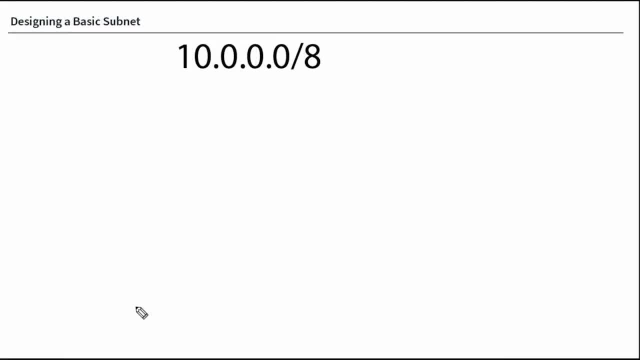 these problems. We've got a lot of stuff that we need to do. We've got a lot of stuff that's a requirement of how many users need an IP address And, lastly, we've talked about stability, about not growing it too big and having a gigantic broadcast domain. Now let's talk about one of the 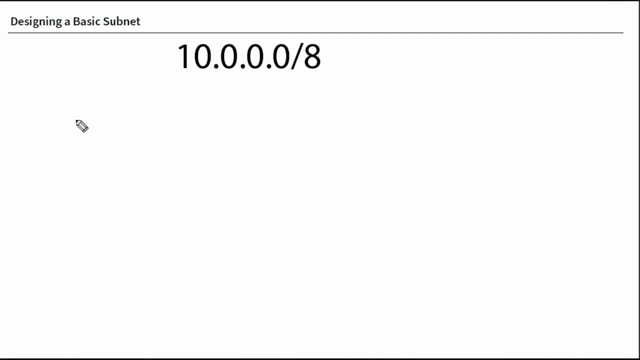 important things that we should consider when it comes to actually designing our subnet. First of all is the gateway IP. It is a best practice to use either the first usable address or the last usable address as the gateway IP. So, to pick on the 10.1.1.1,. 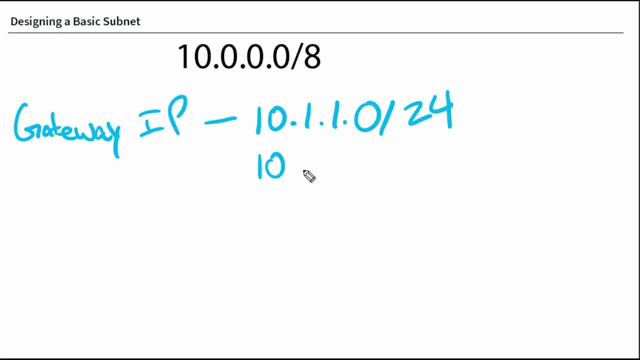 we would want the gateway IP to be 10.1.1.1 or 10.1.1.254.. I don't know why, but I'm so attracted to that 10.1.1.254.. I always thought like, hey, that's really cool. It's kind of edgy. 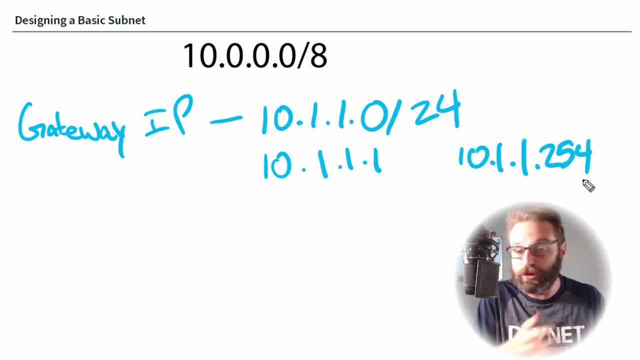 to use the last address And some devices out of the box they really do use the last IP address as their default IP address. It's really up to you and whatever you want to do as a best practice, But whatever you choose, don't use the last bit. 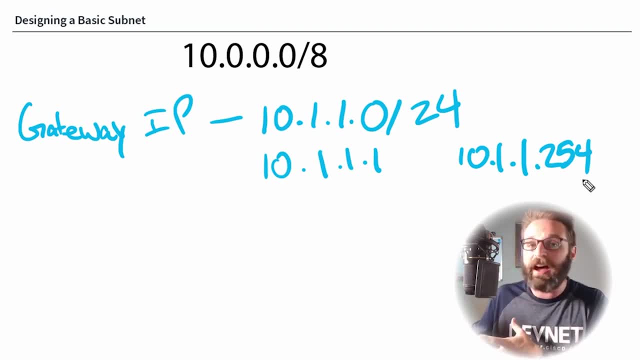 On one subnet and then a completely different design on the other one. If you're going with .254, use .254 everywhere. That way it's standardized and understandable. If you go with .1 as your gateway address, all of your gateways should be .1.. Don't mix it up, because 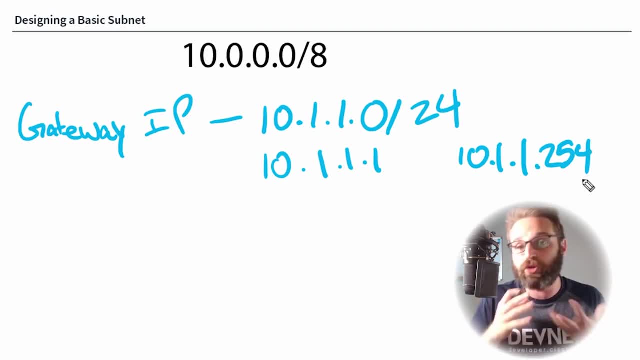 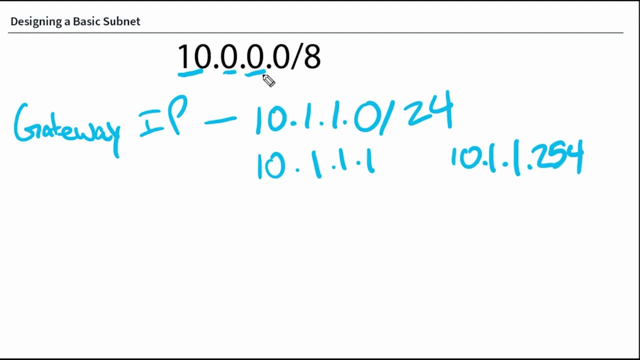 that could be really confusing, really hard to document and really hard to troubleshoot and maintain in the future. Beyond that, we need to pay attention to these octets themselves, because these octets should represent something. Now, the first octet. 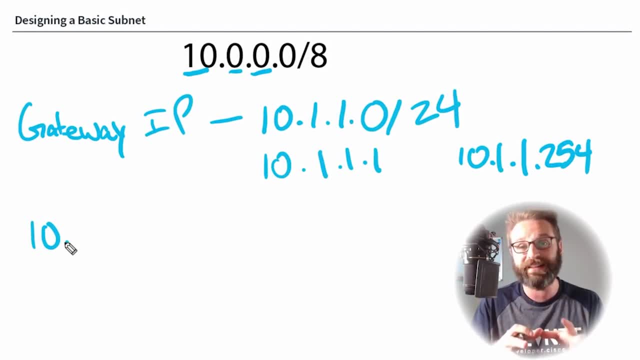 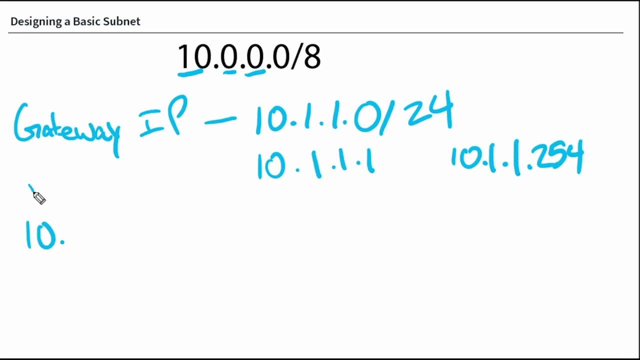 is 10.. Not much you can do about that because that's what RFC 1918 dictates as the actual octet that we need to use for a private address, And people tend to go with 10 so that they can use the other octets to actually represent something In a lot of cases. the second octet actually. 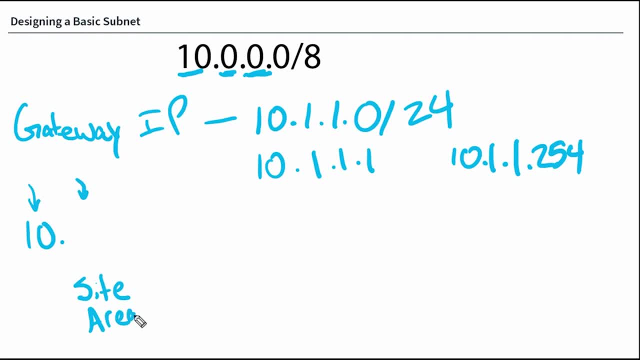 represents the site or the area or some sort of geographical locations like a continent. And this will make a lot more sense when we get to the next nugget and we start talking about the enterprise campus design. but maybe we have three buildings here. We want this building to be 10.1.. We want this building. 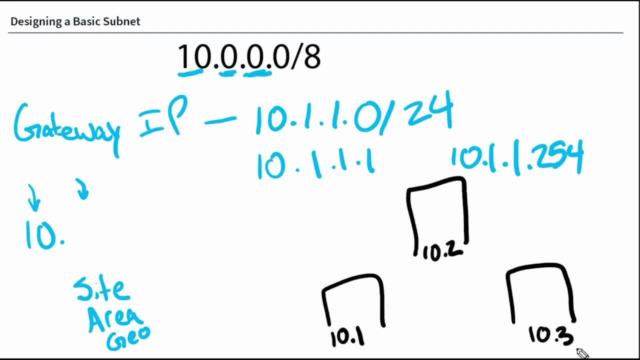 to be 10.2, and we want this building to be 10.3.. So in this case, if I were to set this to one, when somebody reads my IP address and they see the scheme, they would know that this one is. 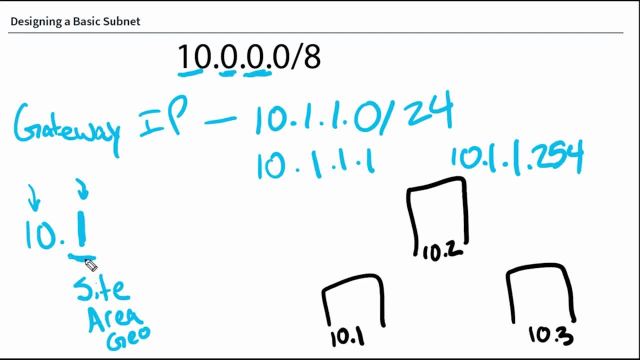 representing where in the world this actual IP address or this subnet is going to be located. Then the third octet here, almost always, is going to represent the VLAN. You see, within these buildings we may have multiple addresses or subnets for data, IOT server and so on, And all of these will exist on different VLANs. 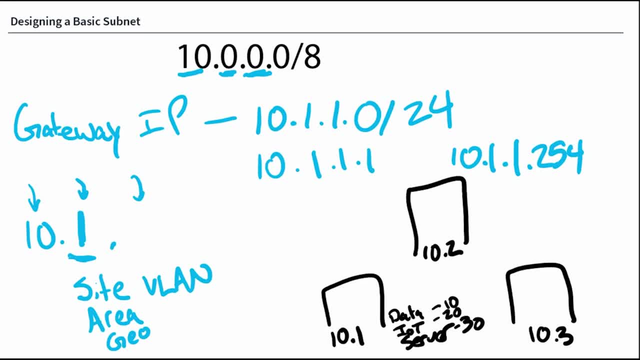 like VLAN 10, VLAN 20,, VLAN 30. So when I set this address to VLAN 30, I see now the okay, this is my private address, It's in building one and this is VLAN 30, which, if I look right here, that means this is my server subnet. 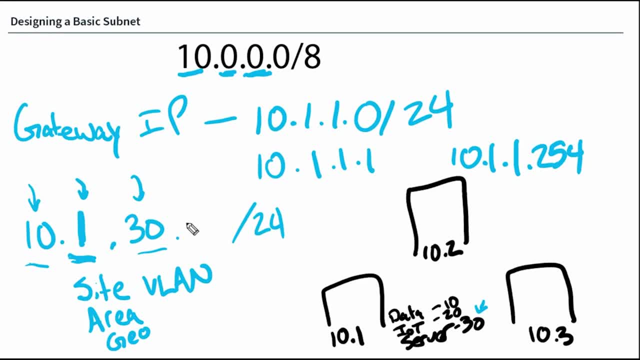 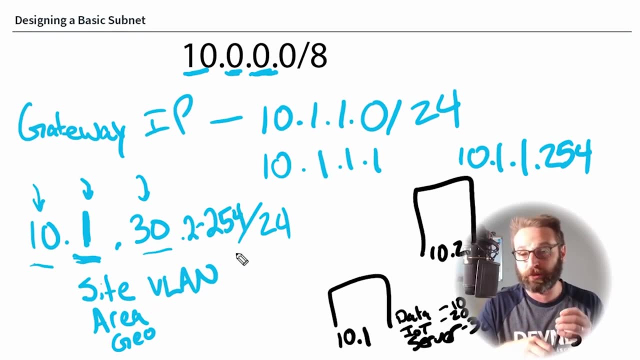 And then if, since we chose to go with a slash 24, we know that the addresses that are available to me are going to be the 253 addresses, So maybe my gateway is one, so my usable addresses are going to be two through 254.. So the basic subnet design is now in place. We've considered the scalability.